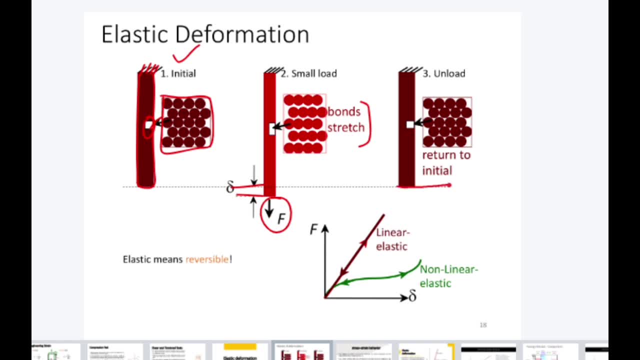 if we remove the, the load again, right now, we have removed the load, this load we have removed, and again we see the atoms and we see the, the, the material, if it comes back to its original position. and after removing the load, we also see that the material is moved to the other side of the body. 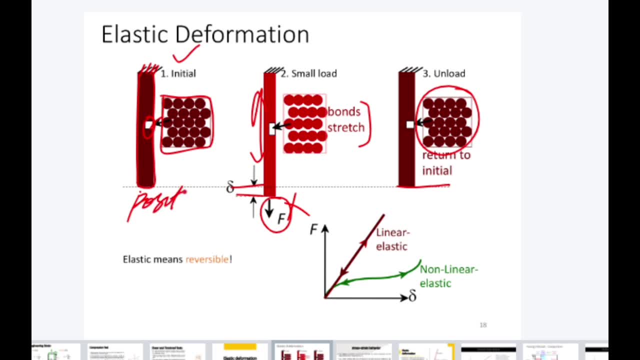 as it was in position 1., Right Position 1. And position 3.. So in position 3, the length of the material is same as the length of the position 1.. So it means the deformation in the material was temporary Right For some time. It depends on the load Once we remove. 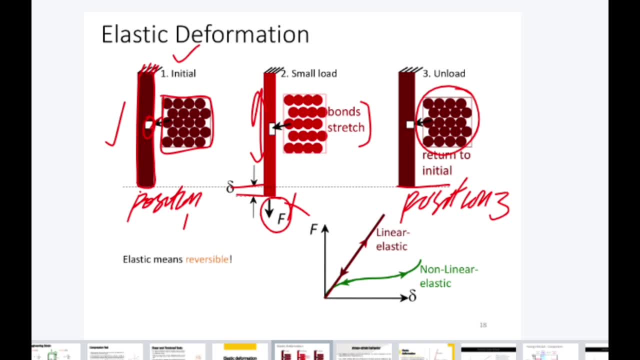 the load, the material comes back to its original state. So this type of deformation is known as elastic deformation. Now, elastic means reversible. We can reverse the deformation. Take an example of the rubber band. If you have a simple rubber band, you pull it and 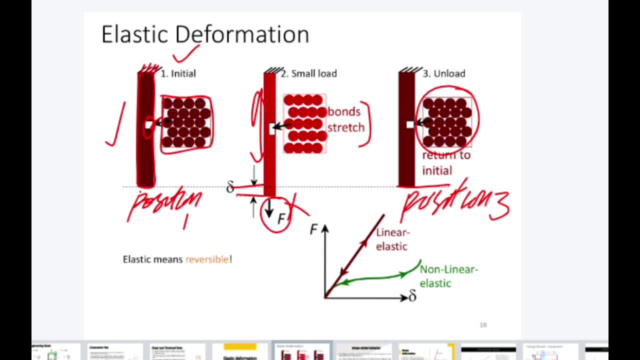 then you release it. What happens? You deform it Right, You increase the length of it, But once you release the load, it comes back to its original position. That is known as elastic deformation. Now, for most of the material, for most of the material, this elastic deformation. 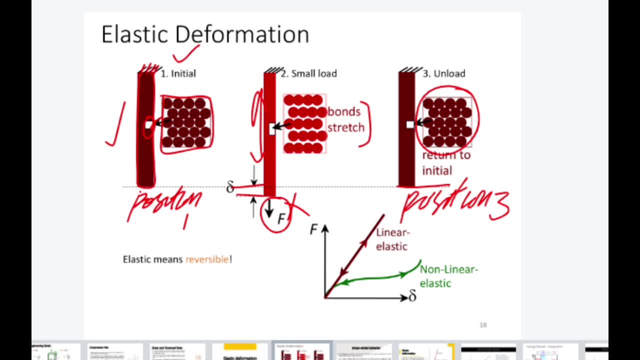 is same. It's linear. What does it mean Linear If we have the strain here and we have the stress here? If I increase, let's say if I have stress, I get the value of strain. Then again, Again. 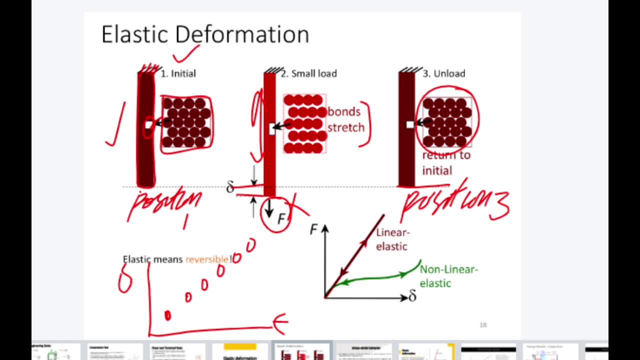 Different value, Right. So as long as I am increasing the stress, the strain also increases. So it gives us a linear relation, Straight line. You see, here This is linear, elastic for most of the material. If you release the force from here, the material will come back. 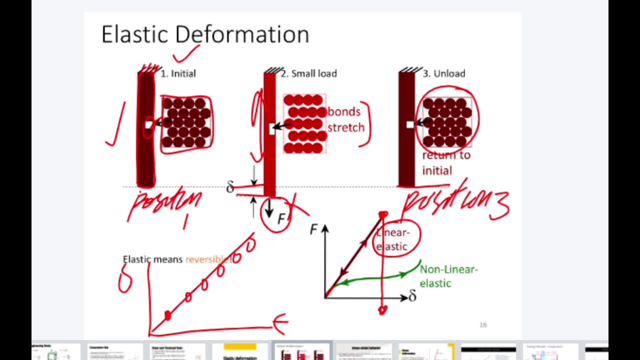 to its original. What is the strain value? This value, Right. But if you release the force, the strain value will come here. So this is linear elastic. For some material, usually for polymer, we see the non-linearity but still there is elasticity, Right, So there is like very few material for the polymer. 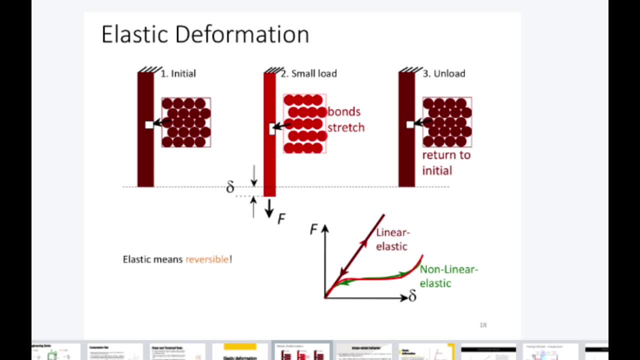 mainly The non-linear elastic behavior we can see. But for metals, for all other, most of the material, we see the linear elastic region in the graph. If you perform this linear elastic behavior, we can see the linear elastic region in the graph. If you perform this linear. 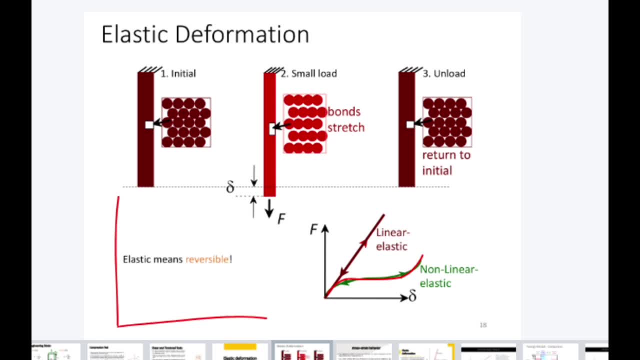 elastic on thesteel Right, With the 개인's test, the concise test, right, and you plot it. so we have the linear elastic region. and then we have the other, this one which we will study later, which is the plastic region, right, This one. We are now studying this region. This is the 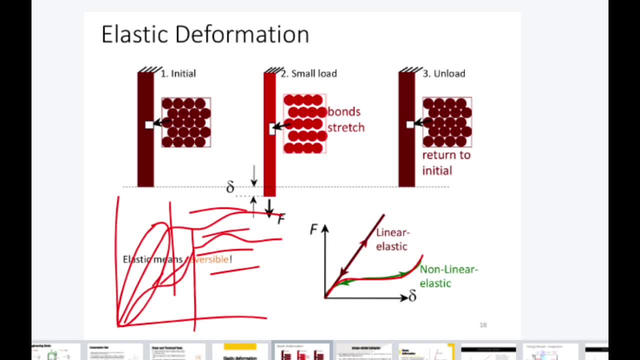 linear elastic. But for some material this region is non-linear But still is elastic. If you remove the white, the film up here and we have the strain here, then the material come back its original position after, In this case after. So we have the linear elastic. 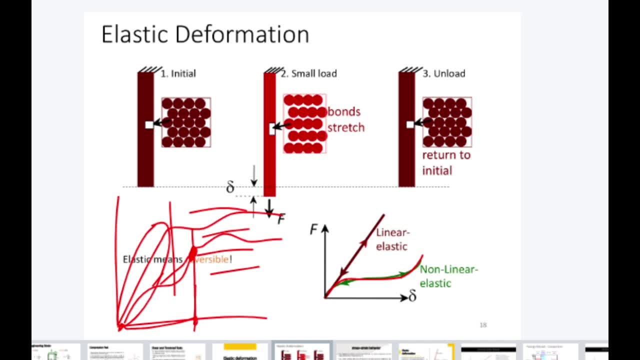 we have the non-linear elastic Add. The main thing for the linear and non-linear is sorry for the elastic. it is like it is reversible and we can bring the material back to its position. Now look here we have the stress-strain behavior. 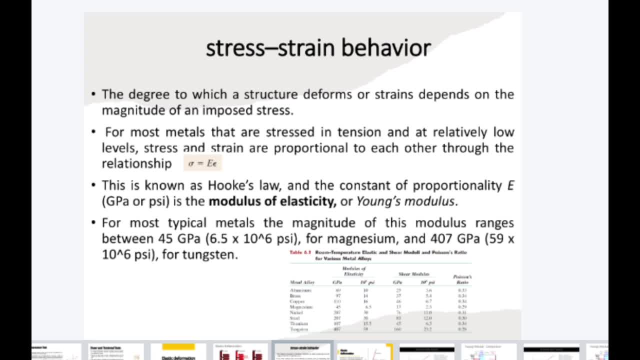 This is. I think I have discussed it. but let us see: The degree to which a structure deforms or strains depends on the magnitude of the imposed stress, of course. Whatever stress you are applying on the material, and then how much it will deform, then deformation. 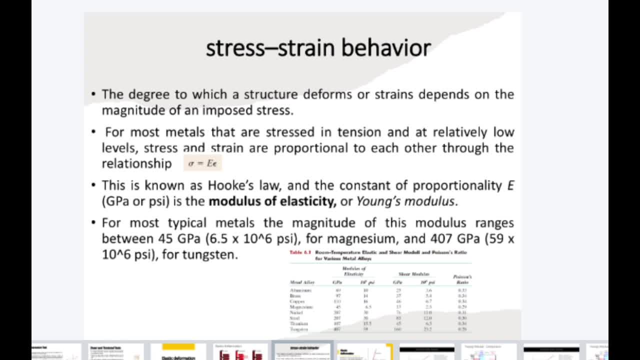 and how much strain occurs in the material will be depending on the stress. If more stress, more strain, More less stress, less strain, For most metals they have stress and tension right at a relatively low level, So the stress-strain are proportional to each other through a relationship which is: 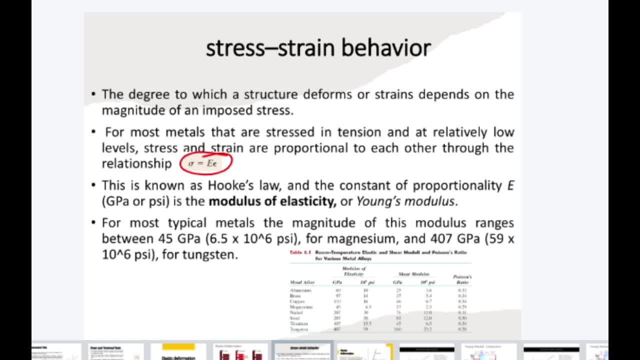 here Sigma is equal to E epsilon. Now this is known as Hoag's law and the concept of proportionality. E is the modulus of elasticity or young modulus. So if we plot it right and in this region we have the strain and stress, 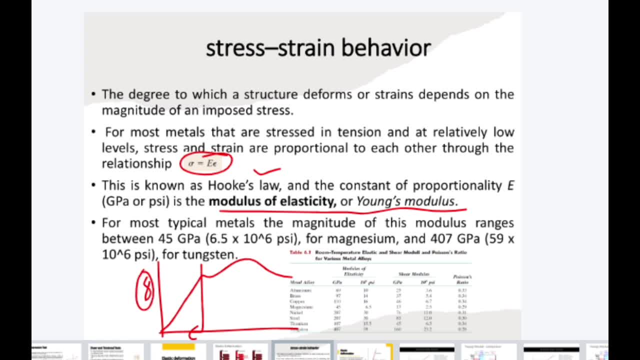 And if we take the relation between stress and strain is like stress is directly proportional to strain. But if we want to remove the proportionality, so we will put the concept of proportionality, and that concept of proportionality is the young modulus or modulus of elasticity. 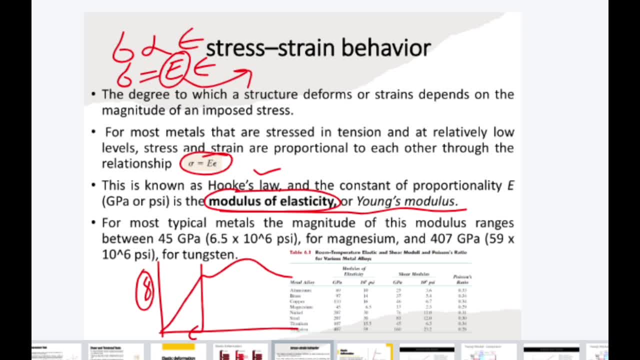 Guys, what is this, This constant of proportionality? what does it mean? You might have seen this: in the F, equal to KX. in the spring constant, You might have seen that Y is equal to MX plus C. Let's say this C is also everywhere here, but let's say we ignore it. 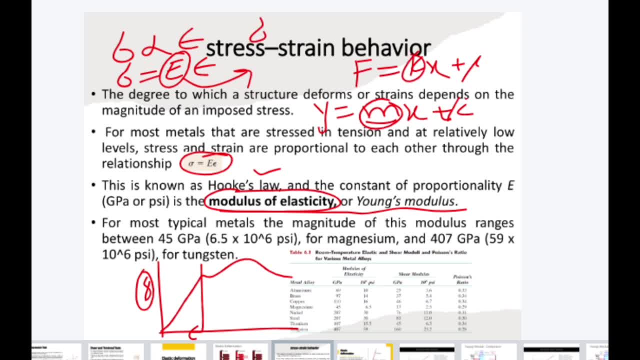 So here we also have the M, Here we have the K, And in this case sigma is equal to E, epsilon. What is this constant of proportionality? What does it mean? It is linear. What is linear Everywhere? you have seen this thing right that we have the linear relationship and then 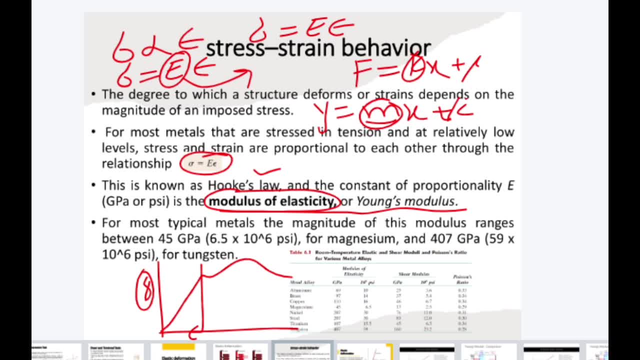 if we find the constant, like even for the acceleration, we have the acceleration, the force is equal to MG, right? So this mass is the constant of proportionality. Now, what is constant of proportionality, Like why it is constant? 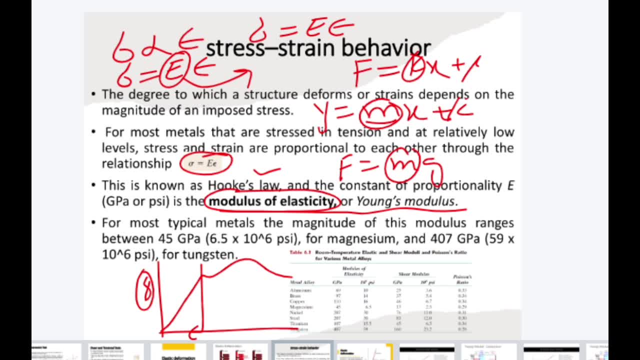 How it is constant. What does it mean? Have you think about it? If you understand, it is good. If you don't understand, just tell me, Because everywhere you have seen this right And you might have Wrote in the exam and everything. 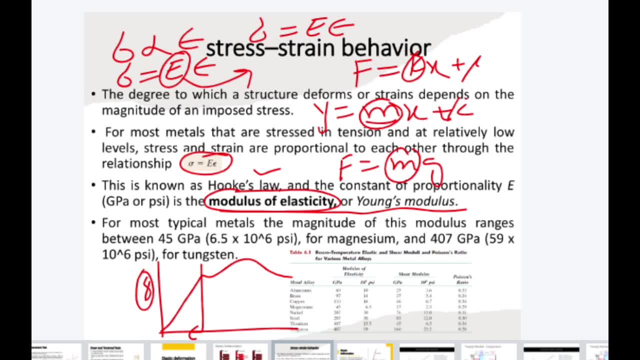 Like the constant of proportionality, and we have a constant here. Now, how? what is constant? What does it mean? Take it truly: Change is linear. So change is linear. That is okay. Then why it is constant if there is change? 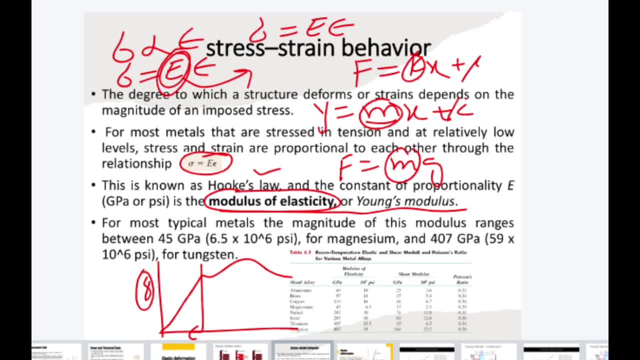 Why we call it constant, This E. we say that E is the constant of proportionality And usually this E M K. if you take the slope of the line, you will get this one right. It does not change. 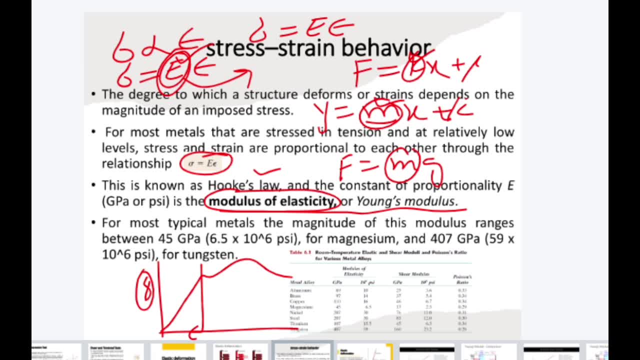 Of course, if it is constant, it does not change. Yeah, you are absolutely right. right, But look, this means what does it mean? If we have a plot, right, Not even for the strain versus stress, right? 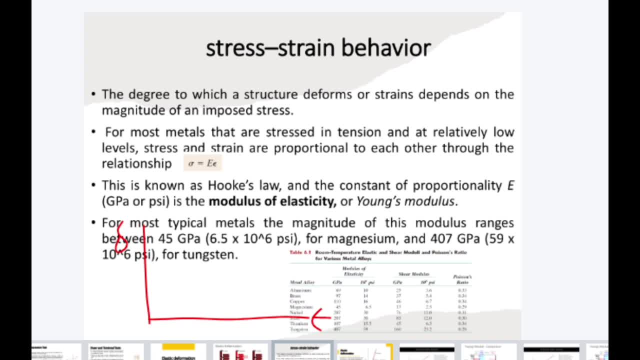 Stress versus strain, For force and acceleration, or force and extension, right, You get a graph And the graph is whatever. it is linear or non-linear. So if we say we are discussing the linear right- Always it is- we are discussing the linear. 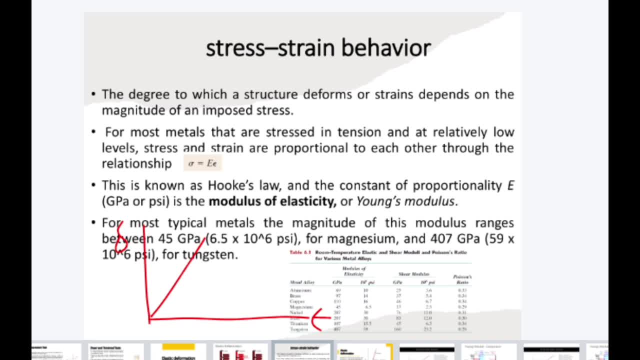 Now, in the linear graph, there is one constant of proportionality. Look into the graph. If it is linear, what does it mean? At this point, I have some value of stress and I have some value of strain. right, I have some value of stress and I have some value of strain. 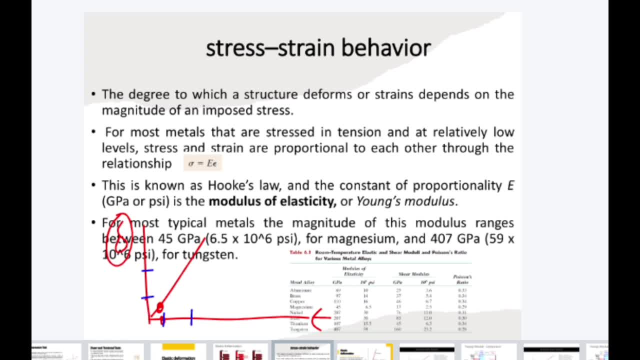 Now, if I take the slope of the line right, If I take the strain value here, I have different value of stress here, Different stress value, different strain value. Along this line, the linear relation, the stress and strain are continuously changing. 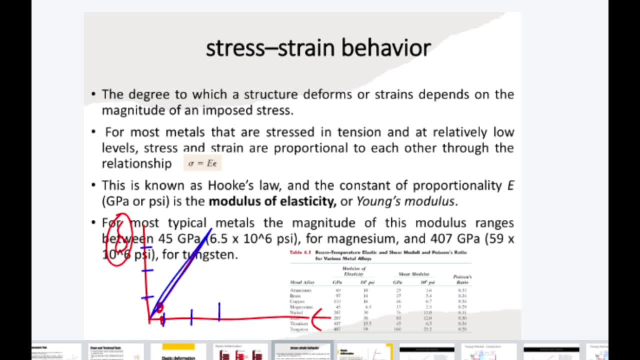 But there is one thing: if you calculate that one thing here, here, here, here, anywhere, if you calculate, that will be constant. That thing is not changing. That is the constant. So in this case, if you find E, 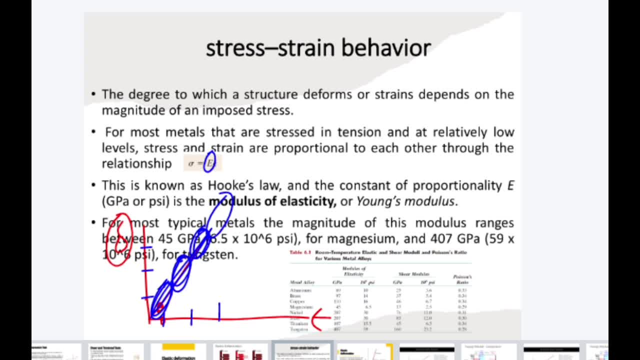 if you find E here, here, wherever, it will be constant, But the stress is not constant throughout the line. Stress is changing, Strain is changing throughout the line, But the modulus of elasticity of E is not changing. That is why it is the constant and the proportionality. 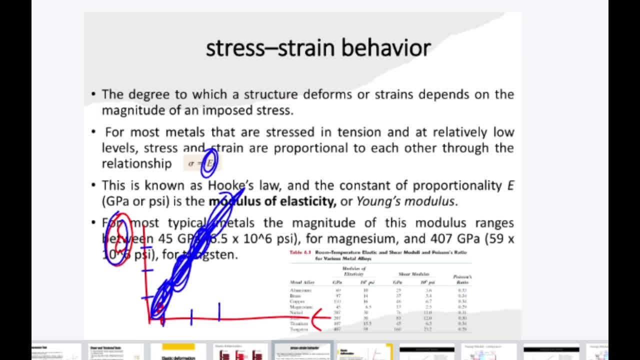 Proportionality means the stress and strain are proportional. If you are increasing the stress, the strain is changing. right. Increasing stress, the strain is changing again and again. But one thing: irrespective of the change in stress, divided by the change in strain, 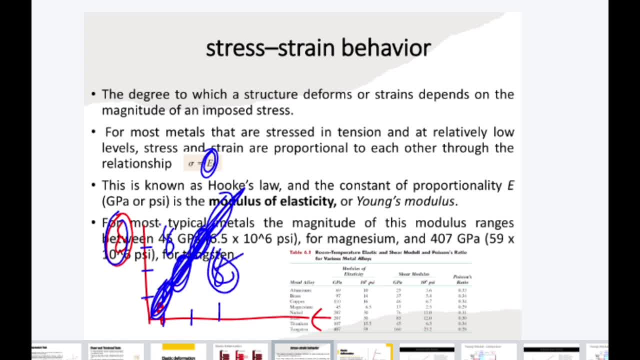 one thing is constant and that is this. E right, It is here. you find here, wherever you find, it will give you the same value. That's why it is constant, And that's why it is the constant of the proportional relation between sigma and epsilon. 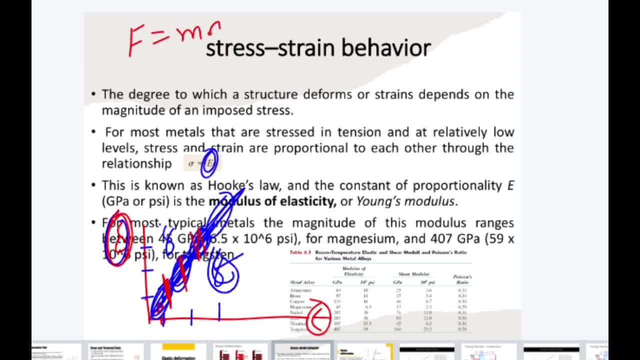 Same for the if we have the F equal M, A. So if we are increasing the force, the acceleration will also increase, right? But if you plug it and you find the slope right, The mass will always be constant if the relation between force and acceleration is linear. 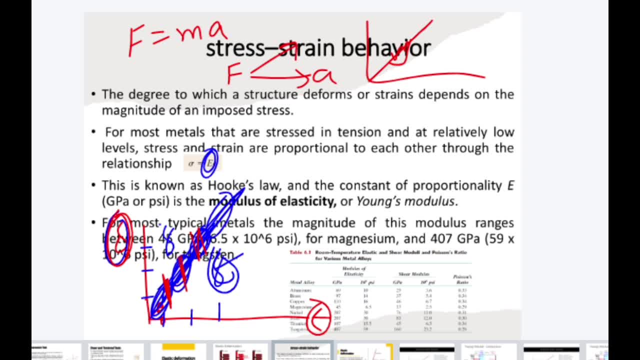 But if the mass, if you are in this case- you can change the mass. If you are changing the mass, then you will not get the linear relation. So that's why here we have this constant of proportionality, and this constant of proportionality is known as modulus of elasticity or young modulus. 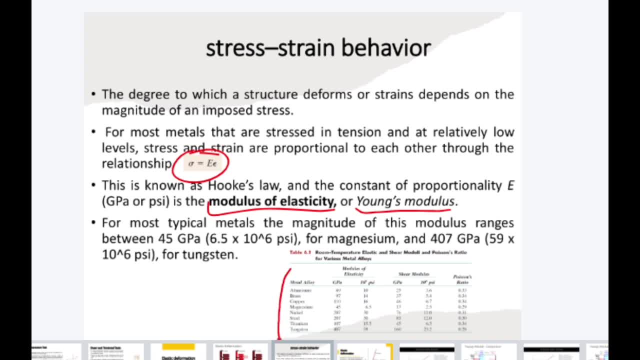 So for most typical material the wave is given for the modulus of elasticity right And the magnitude of this modulus ranges from 45 to 50. It is 5 Giga Pascal R N T S I for magnesium, to 4.7 Giga Pascal for time stamp. 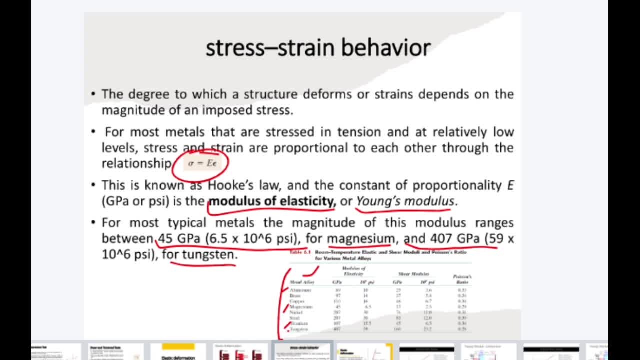 So here is the range for different for aluminum, for all these. Now look, this E is the slope of the line. The slope of the line means if we have this line and we find the slope, and we have this line right. 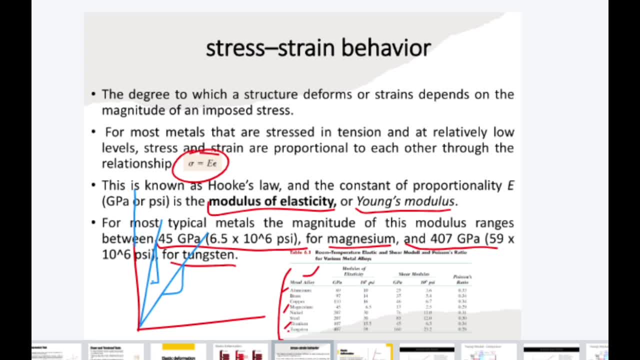 and we find the slope. Now which line will have more slope? Can you tell me, This is line one and this is line two? Which line will have more slope? Two, one. So of course it will be either two or one. 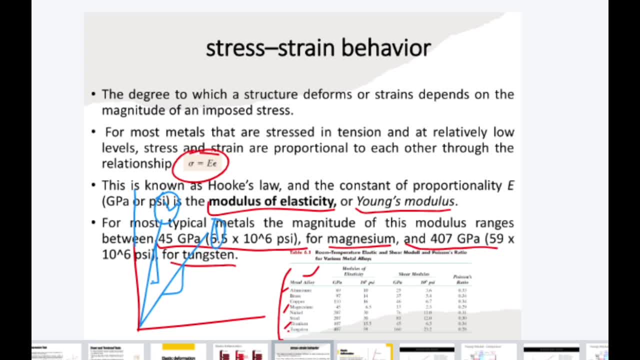 So other guys, please Two. one, I mean two, okay. By writing one, you mean two, very good. So another one is two, okay. Other other guys, Which line will have more slope? Oh, it's okay. 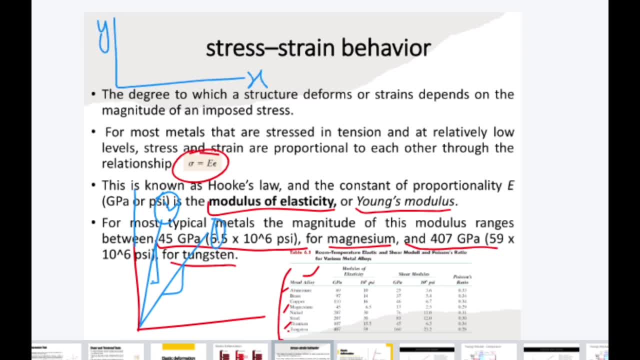 Look now. let's say I ask you, this is the x-axis, this is the y-axis. what is the slope of exactly the y-axis? What is the slope? You have studied math. one right: Infinity. and what is the slope here for the x-axis? 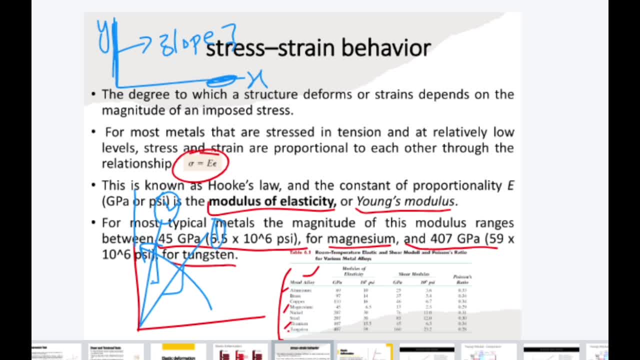 Zero. so it means from here to here we go with the slope increases. So two is right. so line two will have more slope. Now look here from this perspective, from the material perspective, what we are saying If we have a line here. 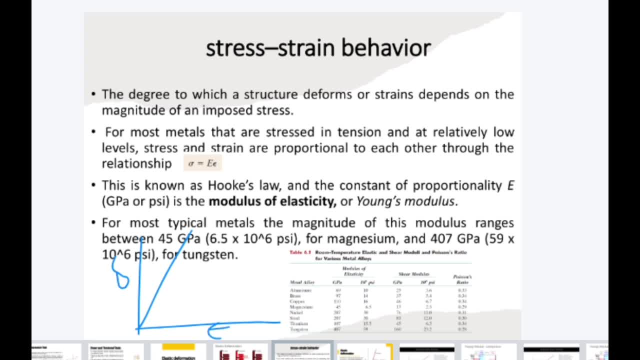 so it means this is the stress, this is the strain. We are increasing the stress, but the strain is not that much increasing, you see, While on the other side, if we have a line like this, what does this line mean? 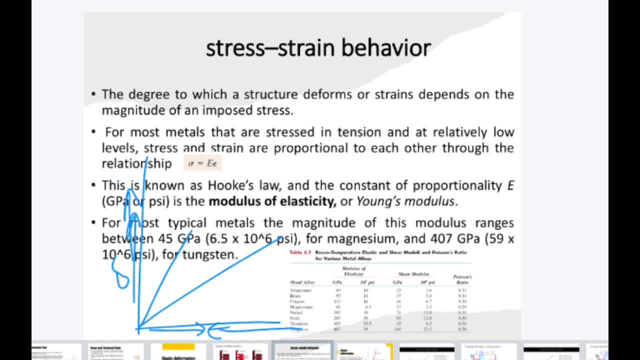 We are increasing the stress a little bit but we see more deformation. So it means the material which have the greater modulus of elasticity. we cannot deform those material very easily Within the elastic region. we are talking right- And the material having less modulus of elasticity. 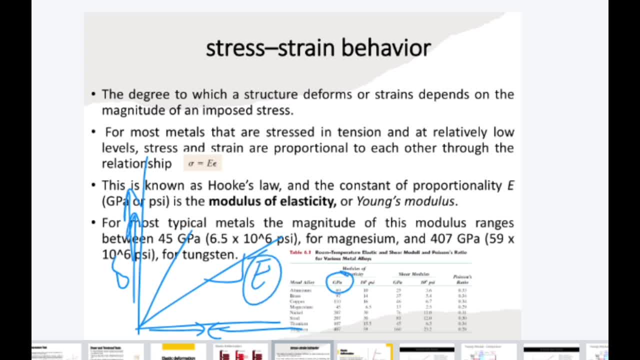 we can deform them very easily, right? This is very difficult to deform. this is very easy to deform. You can see here you might have seen aluminum. Aluminum is soft material, right, Not that much hard, but if you see into steel, 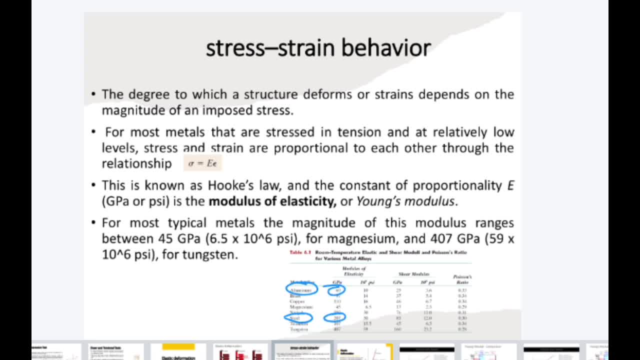 so steel is 207, while aluminum is 69. So now you can understand, right. Like aluminum is soft, we can deform it easily, while steel is hard- like hard, in the sense that we cannot deform it easily, right? 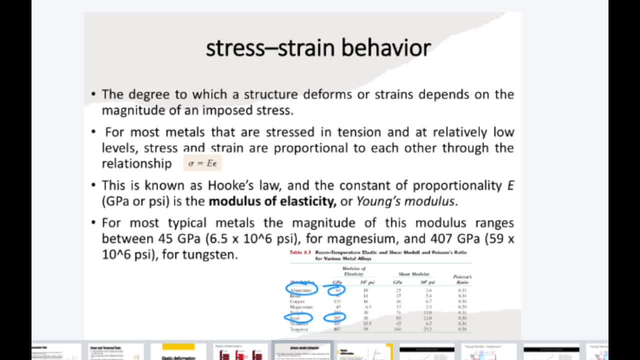 So this is, let me show you right. So this is, let me show you right. So this is, let me show you right. Just like the modulus of elasticity for different material is the order right? 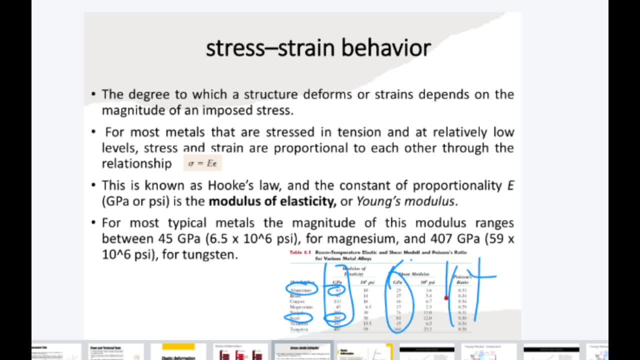 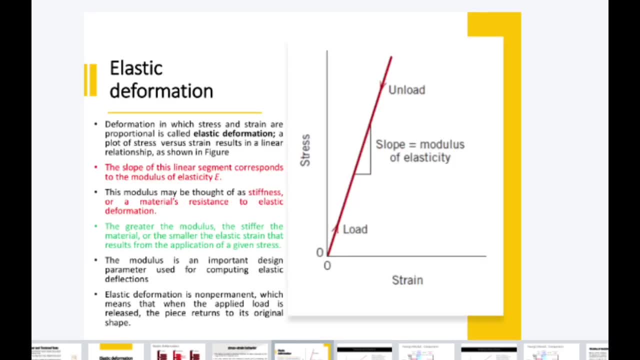 In point them, ratio sheared. the sheared protein has also given The point uncontrolled value we've discussed. We might have stated it in some other course, but he just helped energy production even Now. look here: Yeah, this is the thing which. 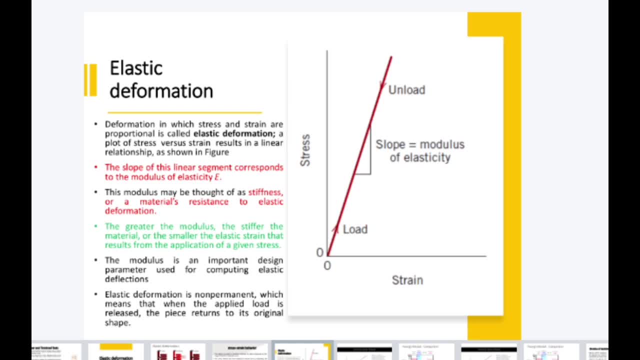 I was doing on the previous slide, We have the elastic deformation. So deformation in which stress and strain are proportional is called elastic deformation. Applied of stress versus strain results in a linear relationship as shown in the figure For most of the material right. 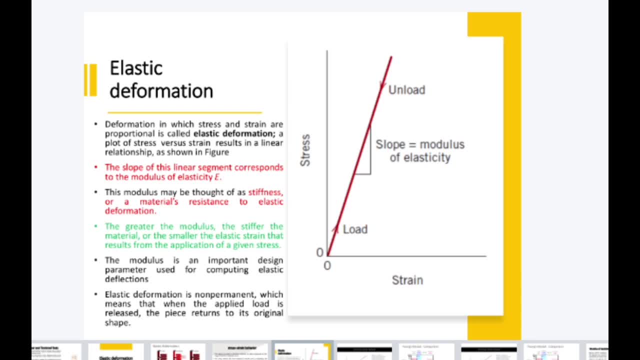 we have the stress versus strain non-linear relation also, but we are not discussing the thing at this level. right, for some polymer we have it. so the slope of this linear segment correspond to the modulus of elasticity. we have this. this is the linear portion right of the graph. the graph is still going there, but we are not taking this into consideration. 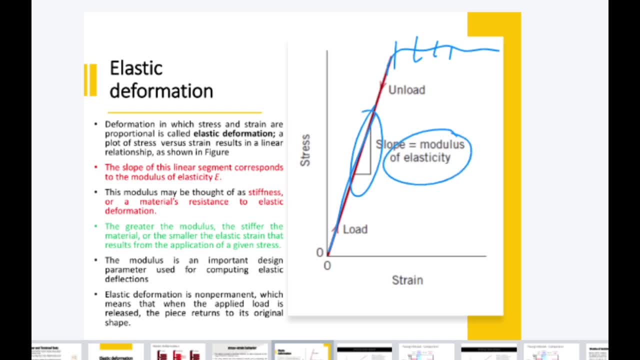 if we point slope here, it gives us the modulus of elasticity. now the modulus may be thought is a stiffness of the material resistant to elastic deformation, as i told you now how the material is resistant. if material is resistant too much to the elastic deformation within the elastic region, if we cannot deform that material, it means the modulus of elasticity is more. but if 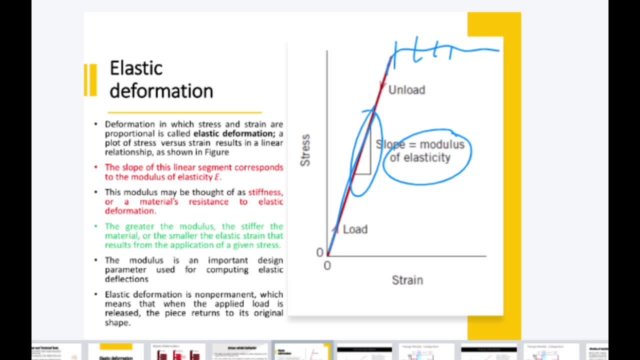 we can deform that material. where is it? it means the modulus of elasticity is less, or vice versa. if the modulus of elasticity is more or less, you can say the same. so the greater the modulus, the stiffer the material and the smaller the the, the elastic strain, or smaller the elastic strain. right. 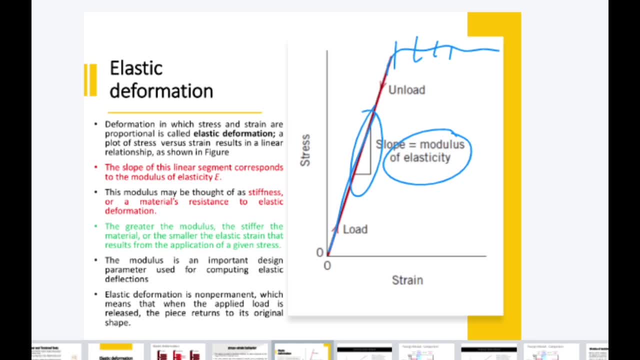 you understand this thing right, very good. so anyone who is confused, this is very simple, right. but you have to understand, like from common perspective, like from a common man, to what you finish the course even so, it should be in the mind: what does it mean if a material is stiff? 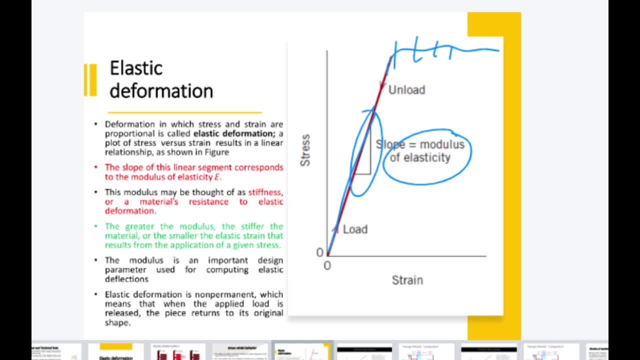 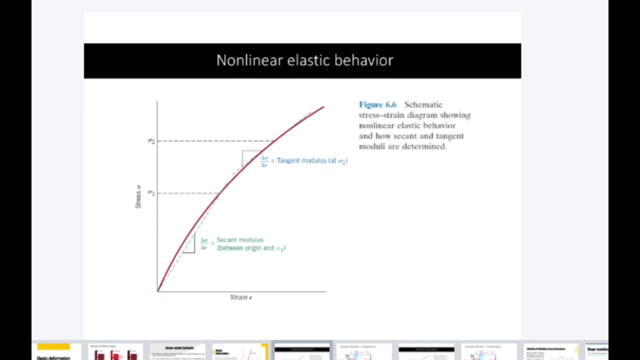 all right. so the stiffness means the material. we cannot deform it easily. if it is not stiff, we can deform it easily within the elastic region. right, clear, okay. now here we have a non-linear glass. sometimes we have in any elastic behavior. the non-near elastic behavior means: now, if you look at this line, it is not linear, it is. 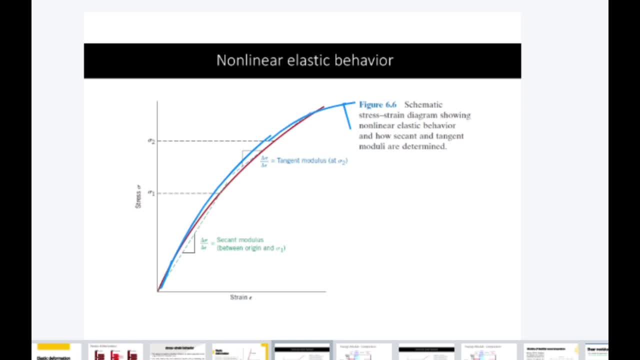 going like this, you see, but what the linear should be like this, but still, this is elastic, how? but some for some material? we see this one, right, we see this one. and if at this point we release the load, so the stress, the strain is this: we release the load, then it comes back to its original position. Now there is another. 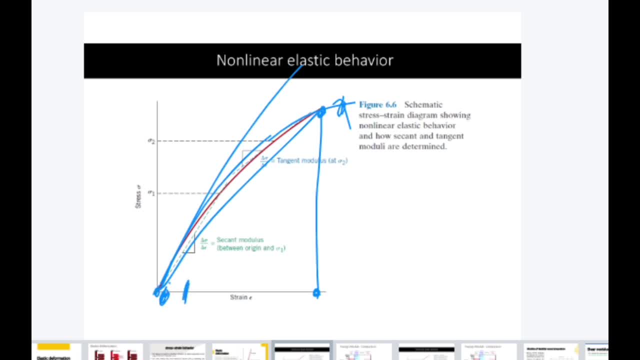 topic. usually it does not come to original position. there is a little bit space, but we will discuss in the coming classes that time right. So for now we are considering that it comes to its original position. yes, So in that case, what we do Now? here we. 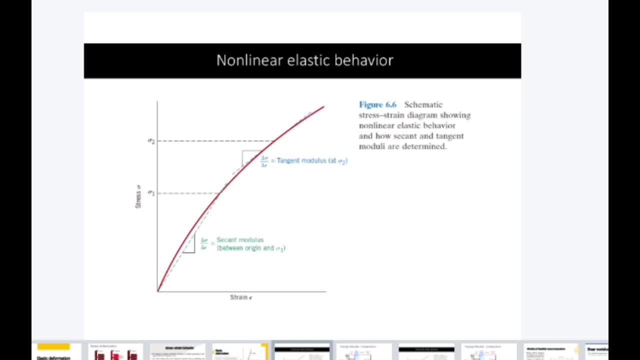 are not finding the scope directly because it is not linear, right? So what we do, we can take two scopes. We can say, yes, this is the tangent modulus and this is the secant modulus. If we have a line, let us say a proper curve, but let us say this is linear. 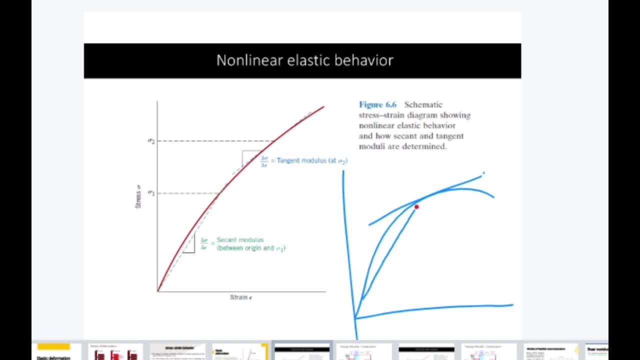 So if you draw a tangent line and if you draw a secant line, right, what is the difference between tangent and secant? Tangent touching one point, okay, yes, okay, good, okay. So secant will touch a two point, So we will. 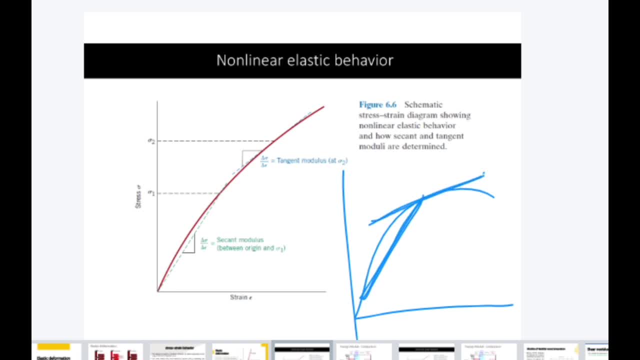 So we will draw a tangent line and then we find the slope. look here We have the tangent modulus, and this modulus we calculate from the line which is tangent to the elastic behavior of the material, and we will do the secant line which will touch the curve at two point. 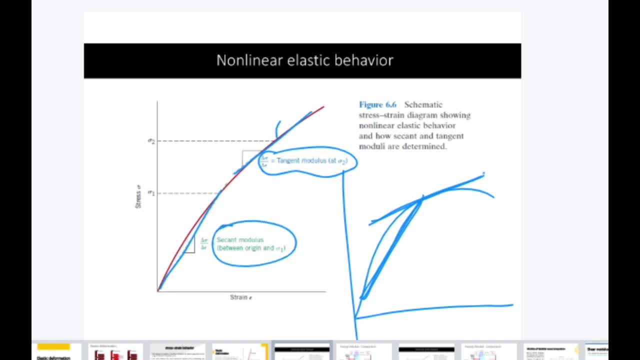 and we find the slope and it will give us the secant modulus. So for these types of material which have the non-linear elastic behavior, we calculate whether the modulus is a secant modulus or tangent modulus. right, But in this course we are not going into. 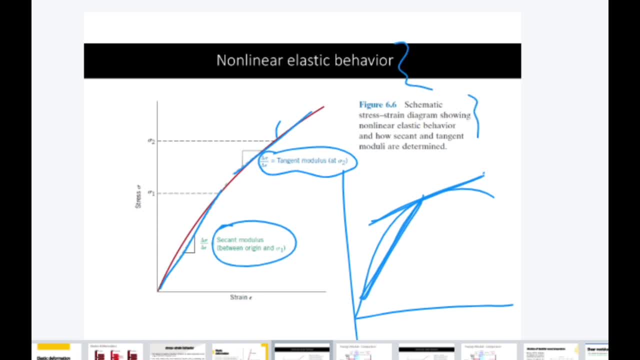 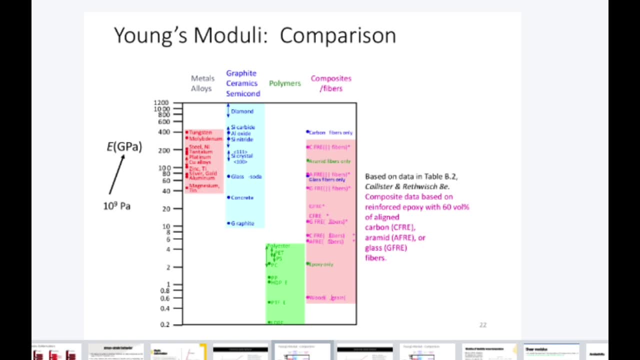 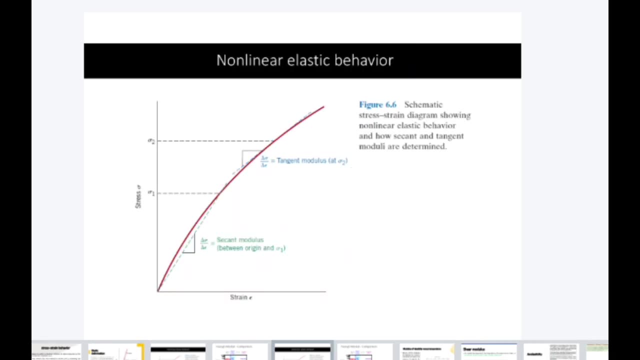 much detail about the non-linear thing. We are interested only in the linear. but just to tell you that this happens right. Clear Professor, does it matter on what point we draw the line? No, look, That is why we do the two right. So if you draw the tangent line here, or if 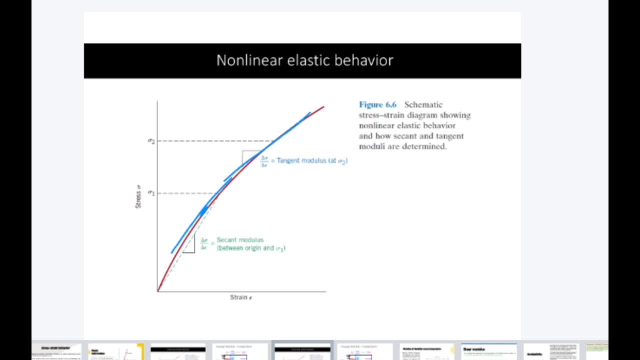 you draw it here right And it touches the curve right. So it touches the curve at one point and it touches somewhere here. So the tangent slope will be the same right And the secant slope. if you draw here here it is not possible even to draw the secant. 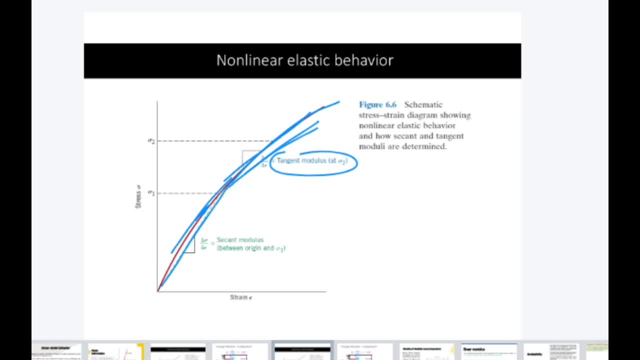 line, because there it is going straight. right. So the tangent modulus and secant modulus. Now is it matter? As can be seen from this line, we can draw only tangent here and secant here, But in some other graph. to be honest, I do not know. You have to search it and tell. 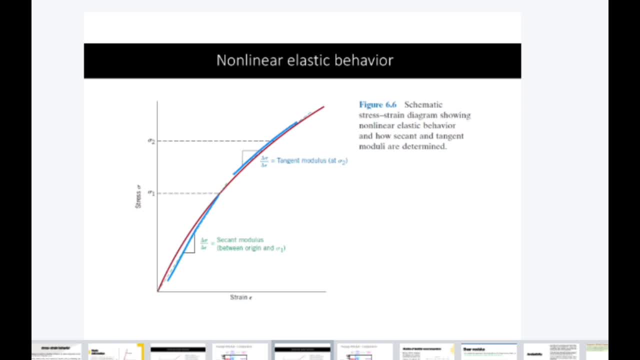 me also What happened. Will it matter or will it does not matter, right? So this thing, better you study and tell me, right, Because we are not going to study the non-linear behavior. So I have not done a lot of work on this, So in the non-linear thing, But there will. 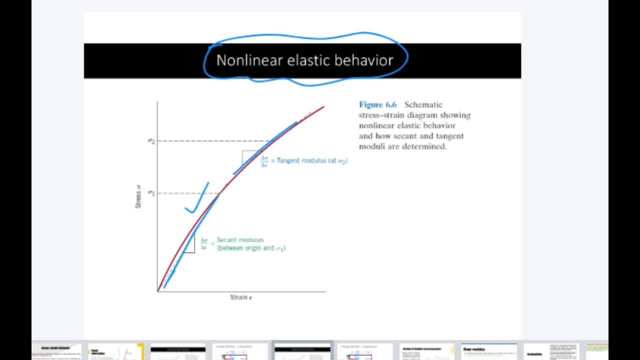 be some answer. You see it and tell me Next class also And I will try to find also. So this is the non-linear elastic behavior. right, We are not going to the details of this one Now. here we have the young models, or the young model of comparison of definite material. 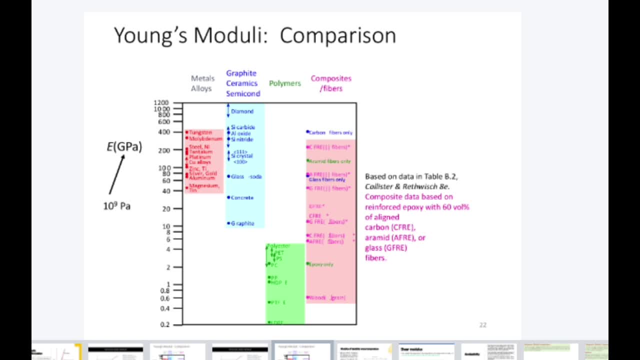 You look here. So this will tell us what. Which material is stiff and which material is not stiff, right? So you see, on the top we have the metal alloys. right, We have the metal alloys. Mostly they have, they are stiff, While in this graphite and ceramic material, 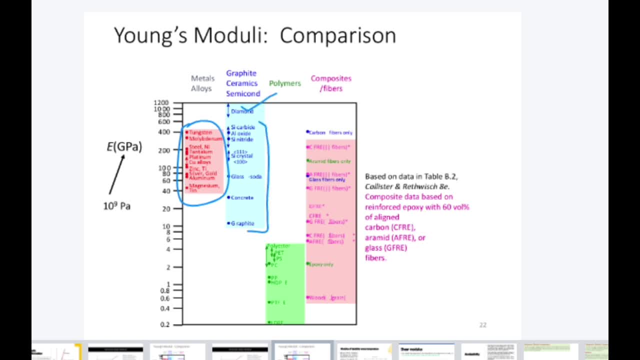 we only have diamond with stiff and the remaining are not that much stiff. The polymers are having the low lowest young modulus while the composite depend. We depending on the composite because composite is something usually we manufacture or we make it synthetically. So it depends what types you are making, right? So for some of the composite it is. 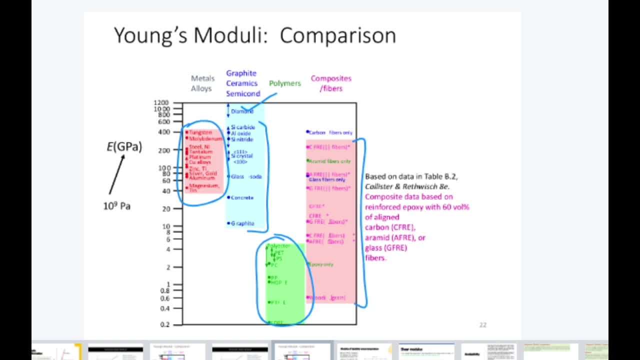 given the value But depends. tomorrow you can make a composite material which is even, let us say, stiffer than all these right, The composite. there are very few natural occurring composite, But all others, what we are studying, are artificial, So we it can. 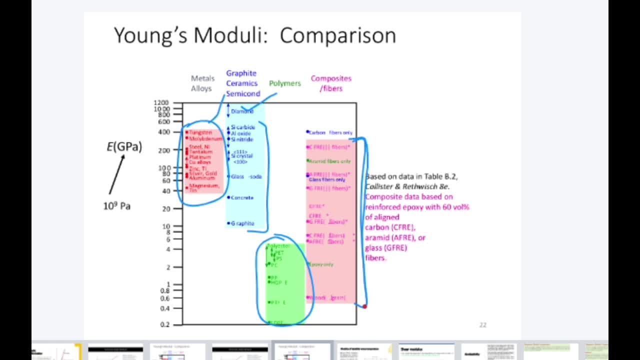 change, right, But so far what we are available are in this range. So diamond is the most stiff material. also, Even it is the most hard material And it is stiffer than all these material, And it is stiff, while then the metal alloys are metal, are stiffer, right, And 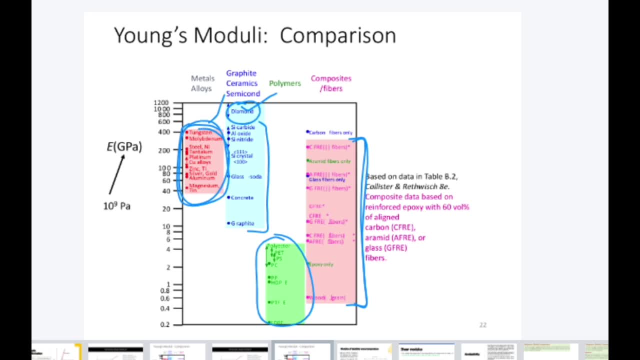 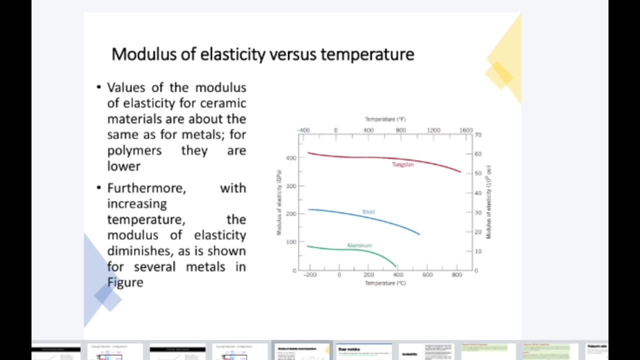 the interatomic bonding has a role in this right, And the crystal structure also. the microstructure also has a role in this. Now the modulus of elasticity. what is its temperature? If we have a material and we change its temperature, we heat it up. So what happens to its modulus? 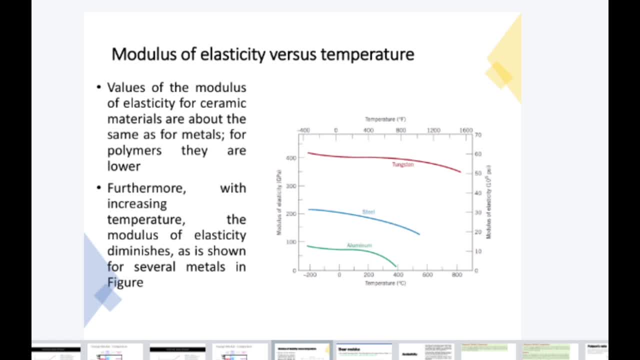 of elasticity. So we have few metals like aluminum, steel and copper. So we have a few metals like aluminum, steel and copper. So we have a few metals like aluminum, steel and tungsten. And we have plotted the modulus of elasticity at different temperature. So 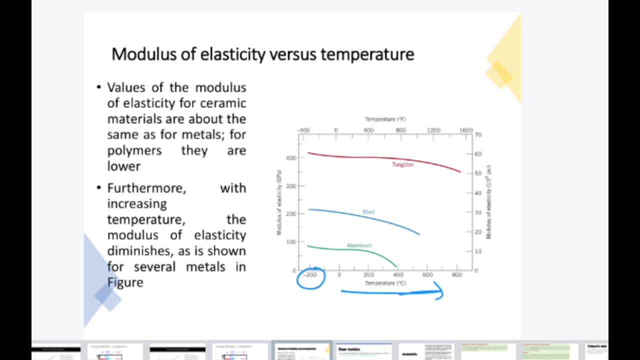 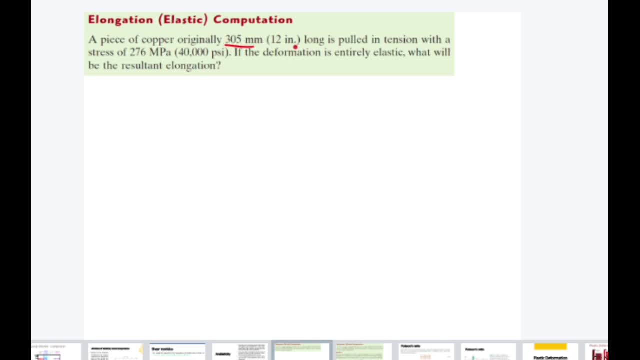 length is 305 mm. It is this much long, right, It is pulled in tension with the stress. The stress is this much: 276 MPa. So if the deformation is entirely elastic, what will be the resultant? elongation. So this thing you have done in mechanics. 2. Now find what is the resultant. 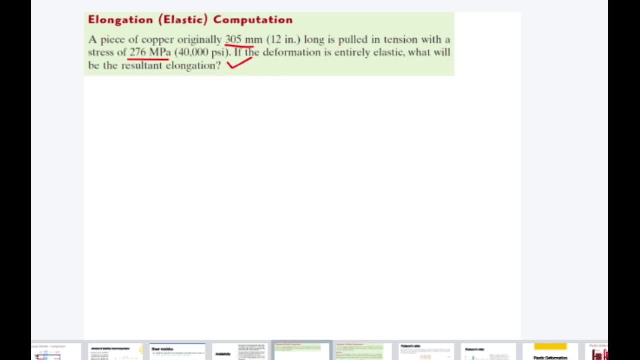 elongation. You are taking this much time. right In mechanics 2, you have a TQ. I have told you what you do to solve the problem. You take data from the statement. So original length is given right. L is given with the 305 mm right. It is pulled with the stress. 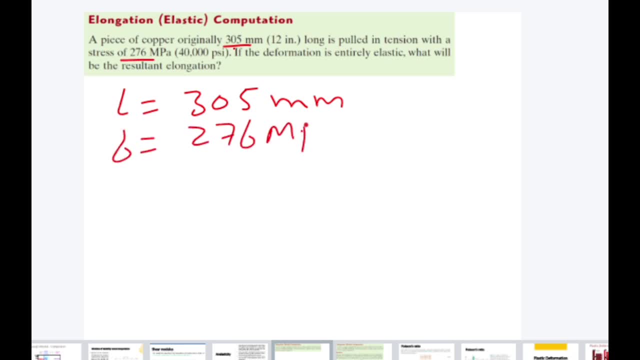 Stress is given, Sigma is given 276 MPa right And we have to find the deformation, the elongation Here. you see, elongation means the change in length we have to find. Now we have the relation that sigma is equal to young modulus or E into epsilon. We can further. 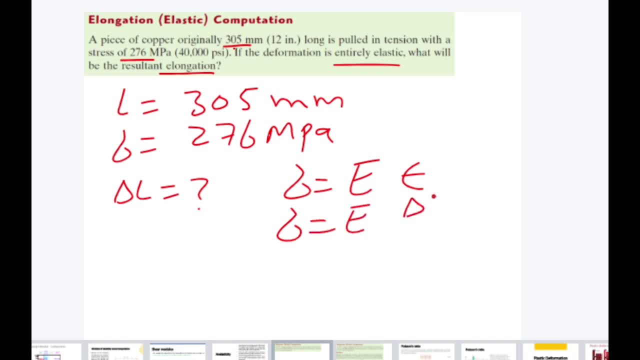 write it. sigma is equal to T. Epsilon is equal to what Change in length divided by original length? We want to find the change in length. So the change in length is equal to what? It will be equal to sigma L divided by E. Now sigma is put the way to 276 multiplied by original length, put 307. 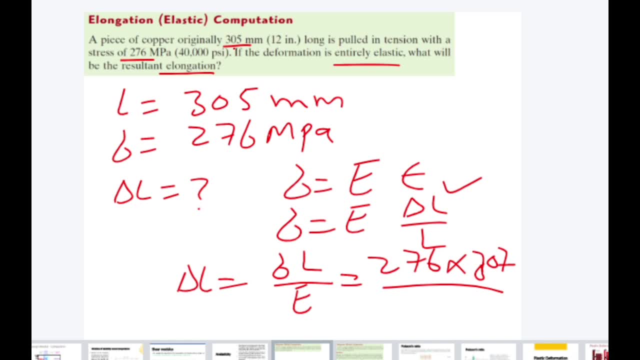 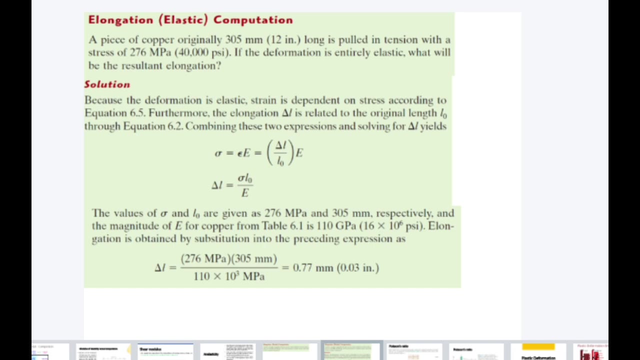 divided by young modulus for steel And before we have our table. But for steel it is usually 110.. So you do all these calculations right. You do these calculations and you will find This is how we do it right. It is not that much difficult Here. you can see, even here. 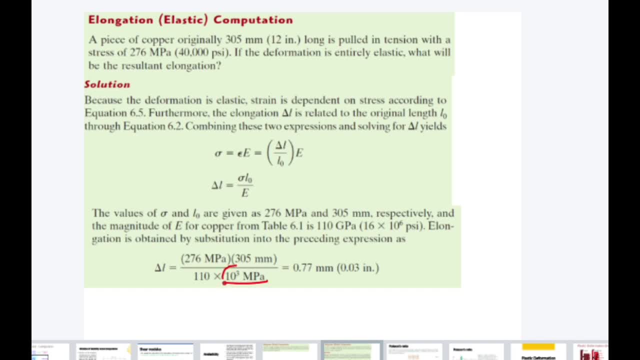 E1. The universe. we can play with it right Now, from Gagapascal. they have converted to Megapascal, So just multiply it, Then this will be power 3. And here also we have Megapascal. 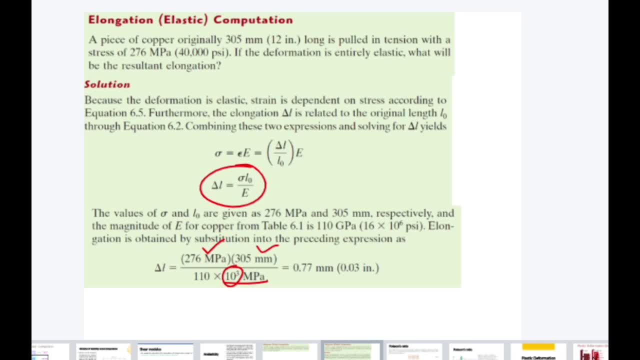 Here we have millimeter, But this is the way of the equation, how we did it right. You can find it. This is not that much difficult. The other thing is we can do it by the energy. So what we can do by the energy, So we can. 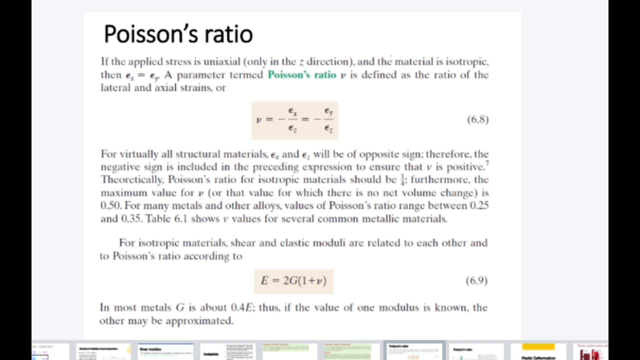 Another thing is the Poisson ratio. this is not like the material thing, but usually it was in the book, so I put the whole slide here. What is it actually If we have a material and we applied a uniaxial stress to the material right? 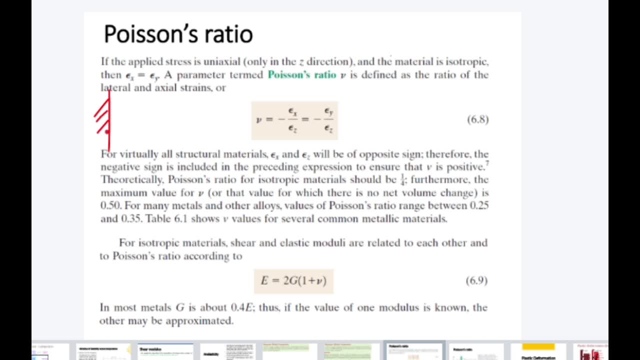 So, like the same way, if you have, let's say, this is fixed and we have the material like this, If this is the x direction and this is, let's say, the z direction, this is the x direction. if we apply a force to this material, it will deform, there will be strain in the material right. 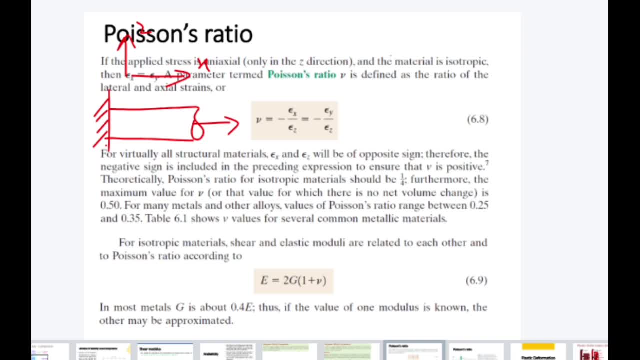 So after deformation, the specimen can be like this. look, it can be like this. So here is a strain in this direction, in the x direction, and here is a strain in the z direction, depending what direction you are taking right. 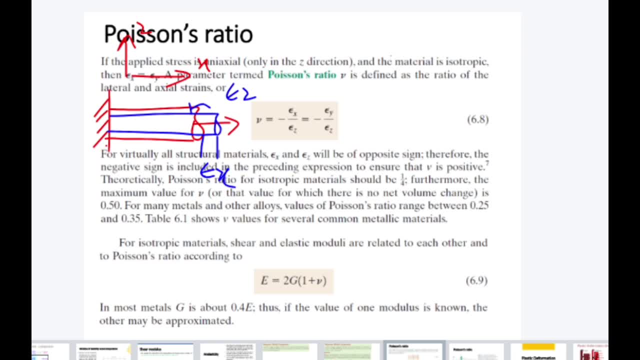 But the longitudinal direction divided by the lateral direction. So if you take the ratio of these two strains, it is will give you the Poisson ratio. Now why there is a negative sign. I told you before, here we are just increasing, here it is reducing. 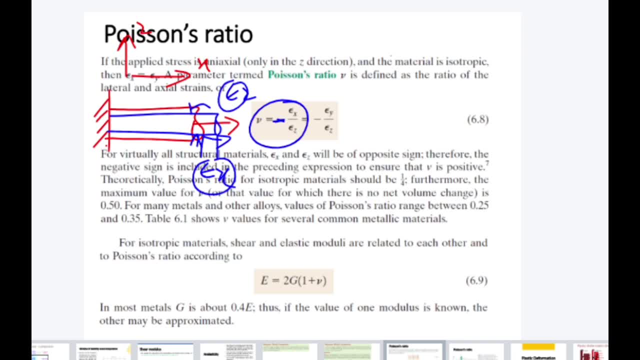 So there will be a negative sign in the calculation and to get the Poisson ratio finally in positive, so we put negative in the formula. So this negative will be multiplied with another negative and finally you will get the value positive. That's why you put the negative sign. 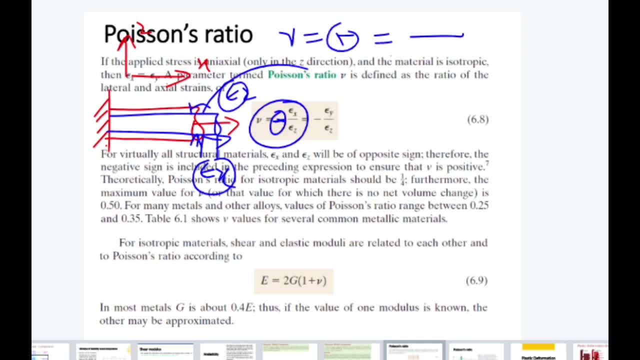 So this is the ratio between two elongation in a material. If you pull a material, it elongates in one direction, the length increases in that direction, while the other direction, the area, is reduced. So the strain in the x direction divided by the strain in the y or z direction, if we take the ratio, it will give us the Poisson ratio, right. 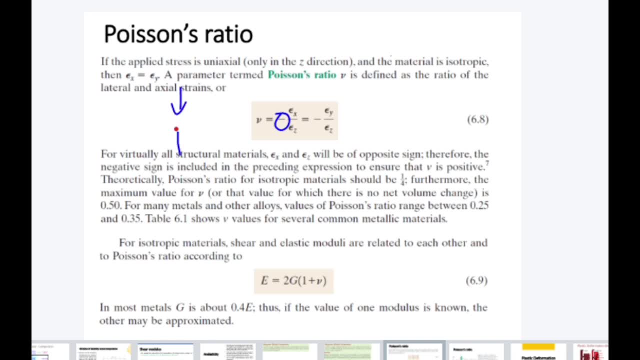 And why we put the negative sign. The negative sign we put because, I told you, when there is a compression, our degrees and the length are decreased in the area. we take it negative. So in the formula and the calculation then we will have negative. Let us say this one is negative or this one is negative. 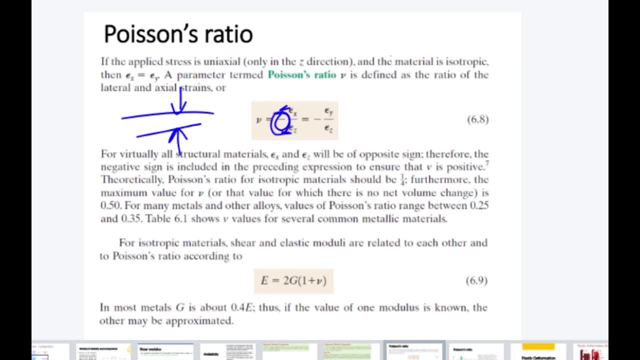 So to remove the negative sign, we put the negative sign before the formula is negative multiplied by negative, then it becomes positive, right? So we get the positive value. You need this whole thing Now. the Poisson ratio is related to the Young modulus and to the Shear modulus. with this equation, right? 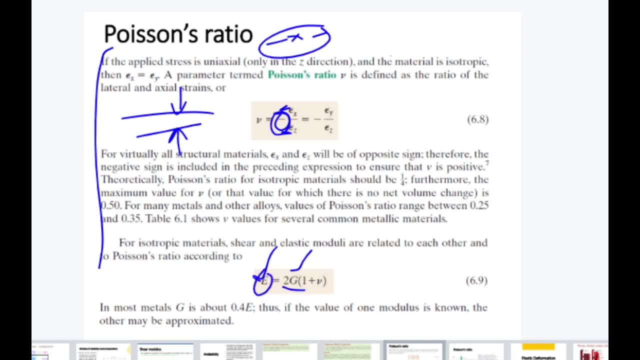 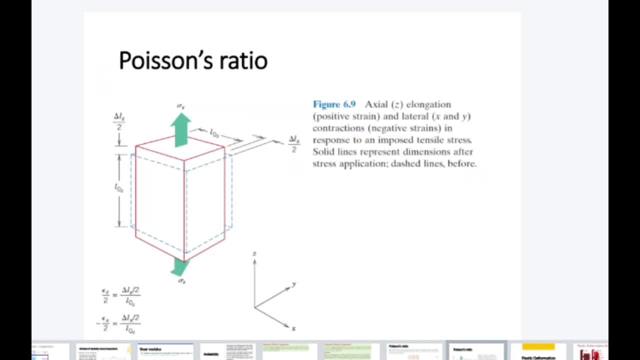 The Young modulus is equal to 2g into 1, plus this italic v, small v, which is the Poisson ratio, right? So this is you just read it. This is fine. Here it is given right A little bit more clearly. We have the force here in the z direction. 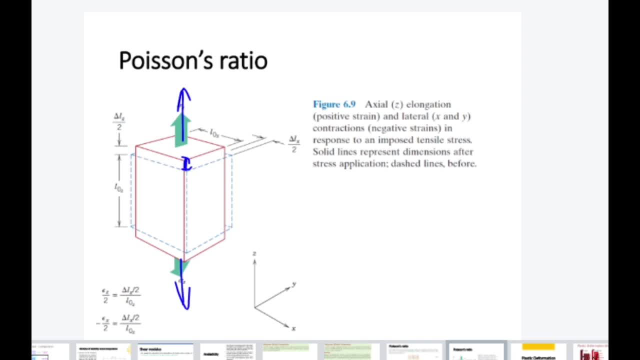 So there is a change in z direction and there is also a change in this direction. So we have to consider both of them and we have to take the ratio of both and it will give us the Poisson ratio. It is simple. 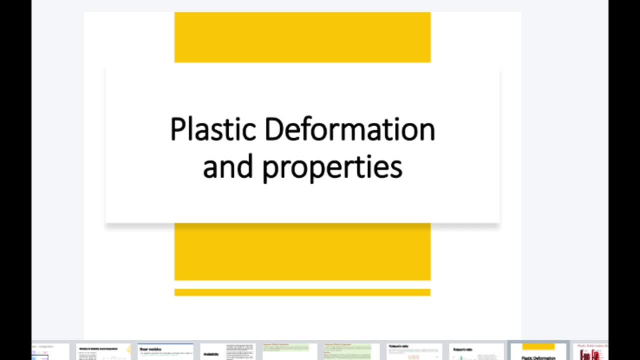 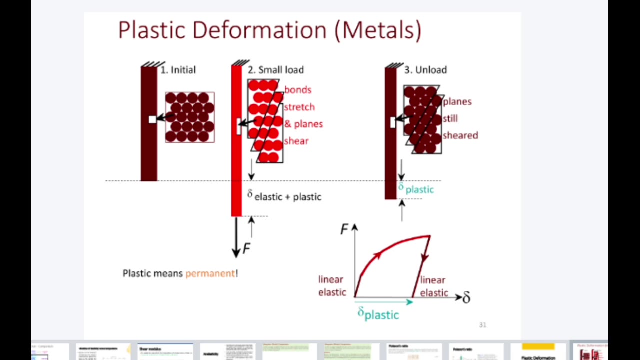 Now we have the Elastic deformation. This is very short and then we are finished, right, We have to start again. Now the Elastic, we have studied, right, But here we have to study the Plastic deformation. Now what is the Plastic deformation? Look here into the figure. It is the same example. 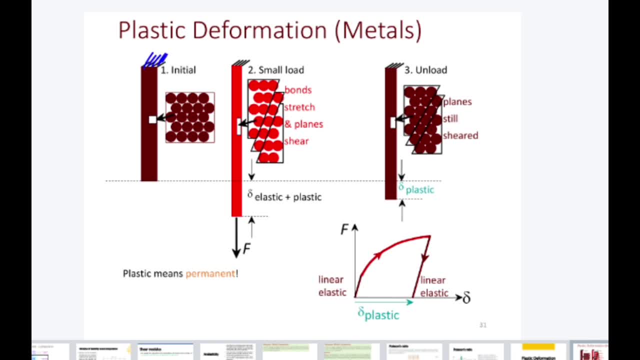 But look, there is one thing: Here we have the same specimen and initially we are not applying the force. So this is the length up to here. This is, let us say, the total length. Once we apply the force, we have the change here, You see. 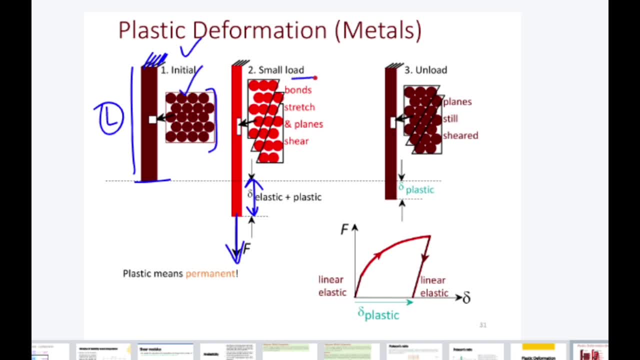 So initially the atoms were arranged like this. Now the bonds are stretched right, The planes are shear. So in the crystal structure we studied there are planes. right There are atoms, One single atom, there are plane. So the plane is shear, right Like this plane is shear. 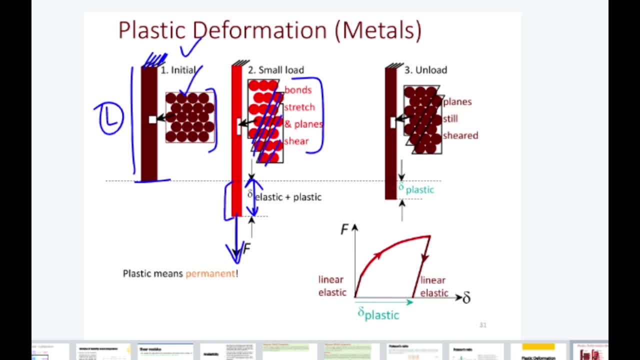 And the bond is stretched a little bit. So that is why we see the elongation, Otherwise we will not see the elongation And then, once we remove the force, the material does not come to its original position. Original position is this line: 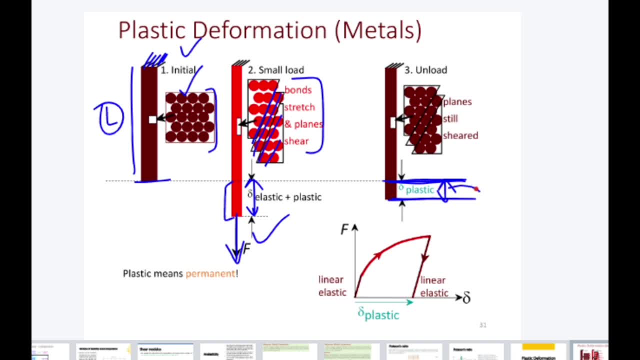 But we see, it is here still. The small change is the plastic change right? So the deformation here, the small deformation, is plastic deformation. Now, plastic deformation means this is permanent deformation. We cannot remove it, Even if we remove the force or the stress, So that deformation is here. 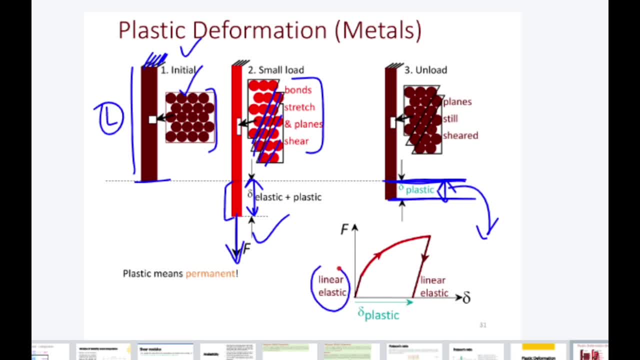 If you look here into the graph, so we have this color, the linear region, This is the force, what is the extension. But if we increase the force, we will reach to one point. let us say this point And then if you remove the force, the strain, the strain will not come to zero. 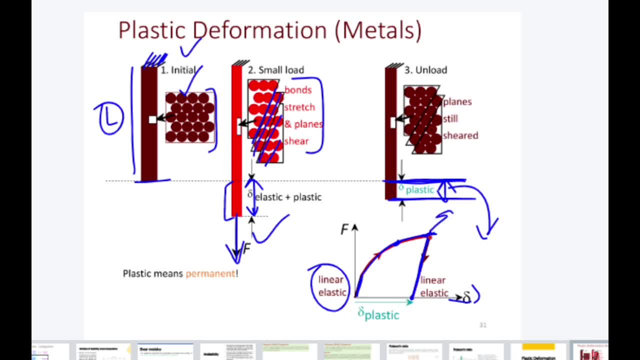 Like if we here, we have removed the force, but the strain value is still here. Let us say the initiator is here right Now. this deformation, or this much strain, is known as plastic strain. You might have experienced this one If you have a soft metal, let us say aluminum or something, if you pull it right. 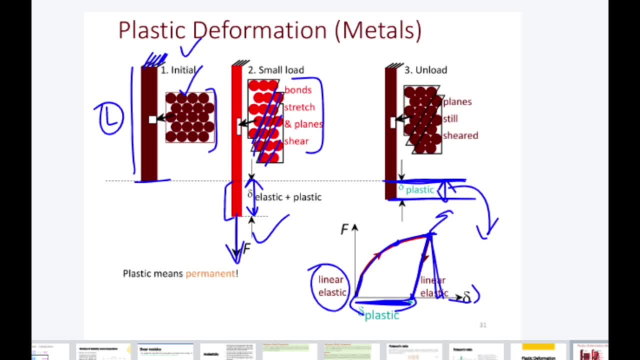 So after some time it does not break, but you see there is increase in the length And it is permanent. Then, even if you release the force, like the rubber band, it does not come to its original position. Why? Because we have crossed the elastic limit and we have reached to the plastic region. 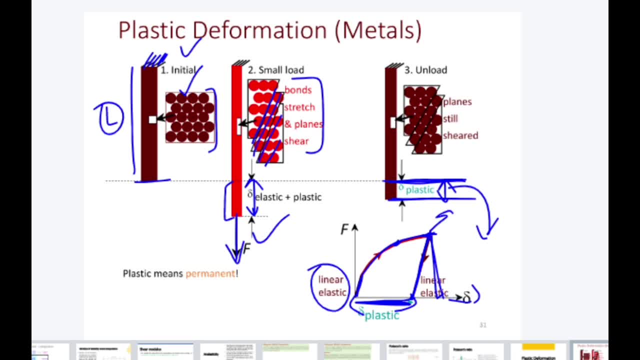 So that deformation is known as plastic deformation. Any confusion From the graph we will discuss in the next class, like this graph in detail. anyone I have discussed in the last video, Like here after here. this is the elastic limit. 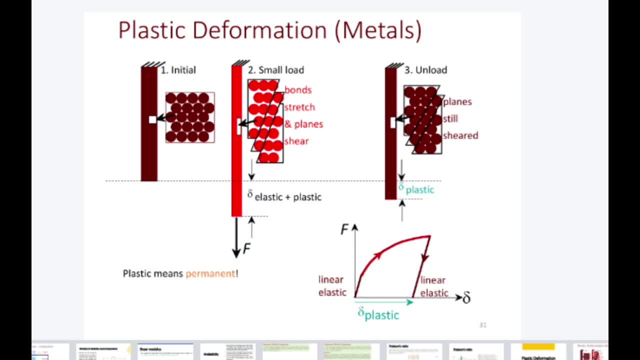 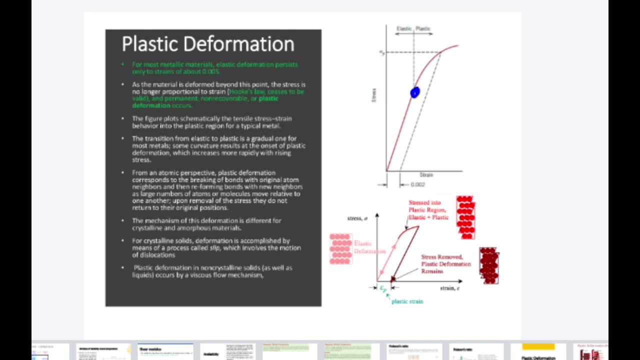 So before this, this is the elastic region. After this, this is the plastic region, And you can see here, even in the graph. Now look here into the graph. This is the point P is the elastic limit, And if we go beyond the point P, we have the plastic deformation. 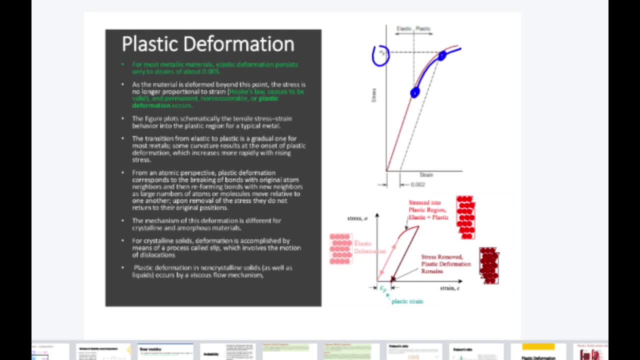 And look here at point P, in the plastic region we have the- let us say- one value of stress If we release the force here. so this strain was here, But if you look here still it is. we have this amount of strain which is the plastic right. 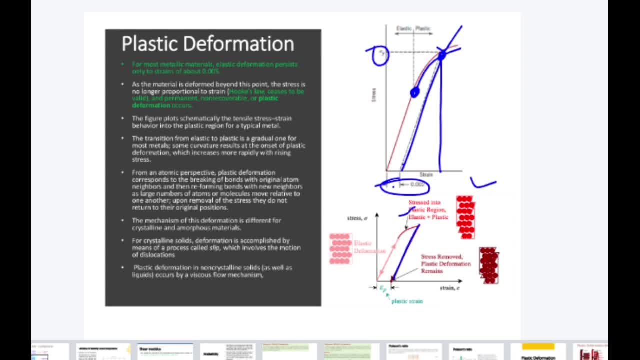 Also, you can see from here, if you release the strain, the stress. this strain should go here if it was in the elastic, But within when it reaches the plastic region, this is not going here And we have this small strain which is known as the plastic strain, right, 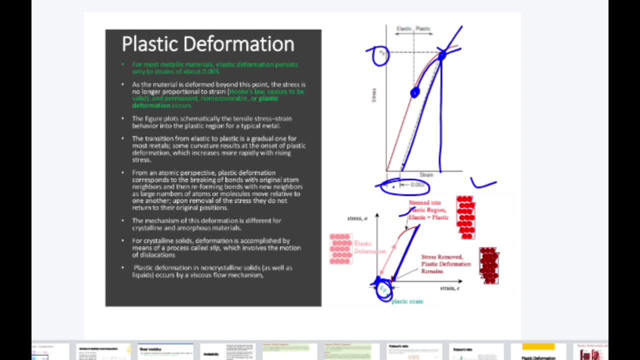 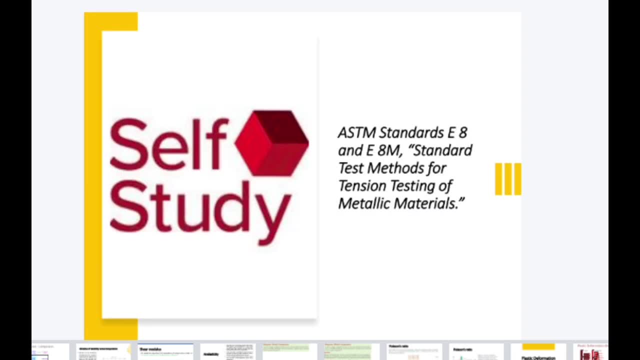 So there is that permanent deformation And that permanent deformation is known as the plastic strain or plastic deformation, Plastic deformation or plastic elongation. right, This theory, you have to study it. there is nothing. And that is it for today.